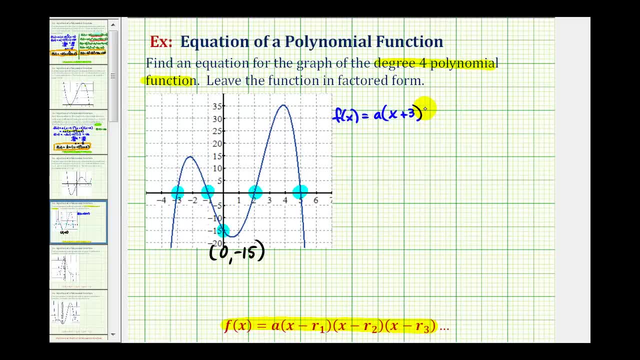 If one of the factors is x equals negative one, then a factor must be x minus negative one or x plus one. Next, if we have a zero of positive two, we must have a factor of x minus two, And if we have a zero of positive five, we must have a factor of x minus five. 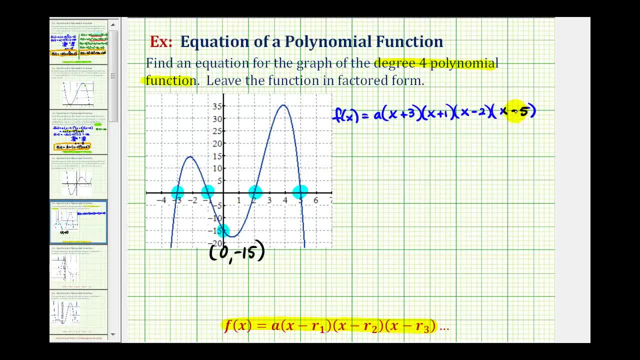 Notice how the constants in our factors have the opposite sign of the zeros from our graph. If we set these values into our function, one of these factors would be zero. Therefore, this product would be zero And the function would equal zero indicated by the graph. 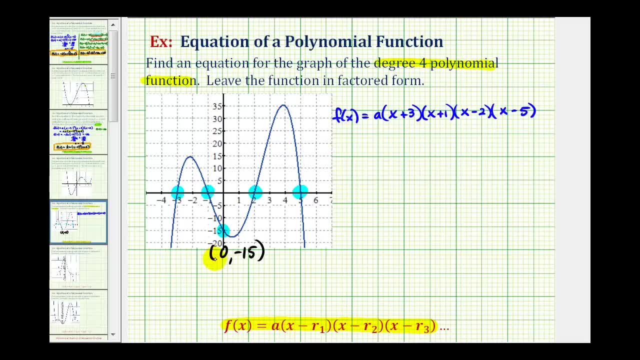 And now to find the value of a. we'll use this point here. If the function contains the point zero negative fifteen, this means f of zero must equal negative fifteen. So we'll substitute zero for x And set this function value equal to a. 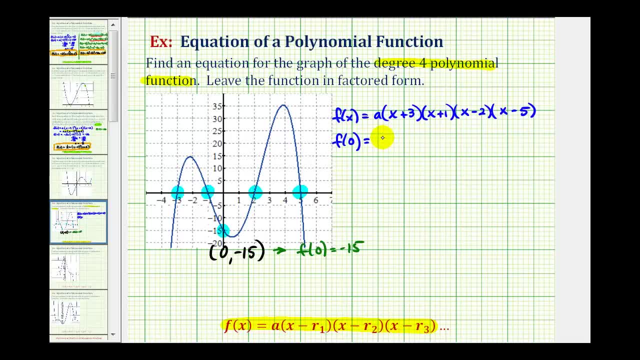 Negative fifteen. So if x is equal to zero, we would have a times three times one times negative, two times negative five, And this product must equal negative fifteen. So now we'll go ahead and solve for a Three times one times negative two, that's negative six. 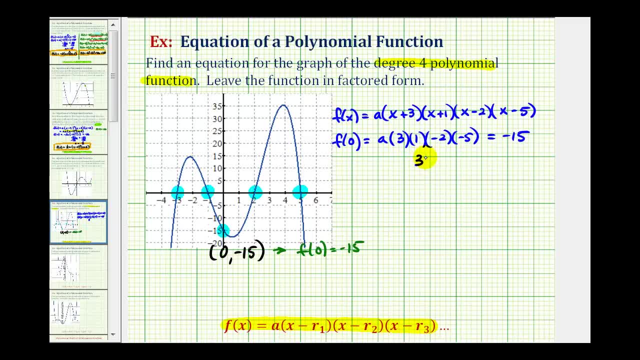 Times negative five is positive thirty. So we have thirty a equals negative fifteen. Divide both sides by thirty, We have a equals. this simplifies to negative one half. So now we have all the information we need to write our polynomial function in factored form. 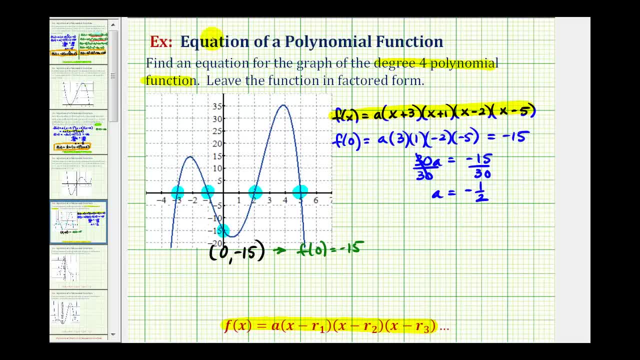 Using this form of our function, we'll substitute negative one half for a, So we'd have f of x equals negative one half times the quantity x plus three, Times the quantity x plus one, Times the quantity x minus two And times the quantity x minus five. 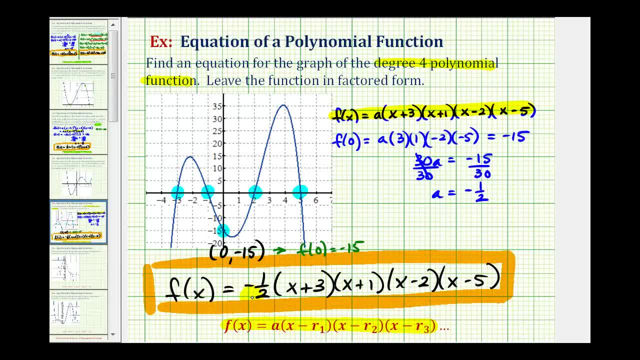 Notice, if we multiplied this out, The leading coefficient would be negative And it's a degree four polynomial function. So notice, as we move to the left and right, The function is going down, Approaching negative infinity in both directions, Which is what we expect.